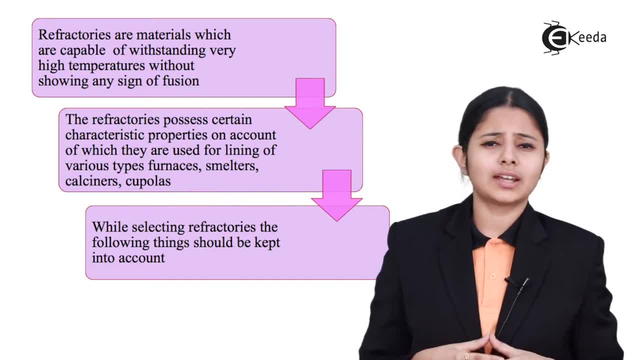 by the virtue of refractory materials. the temperature of the glass furnace is not high. By virtue of the property of refractory materials withstanding extremely high temperatures, they are used for lining the interior materials of blast furnace, crucibles, smelters and. 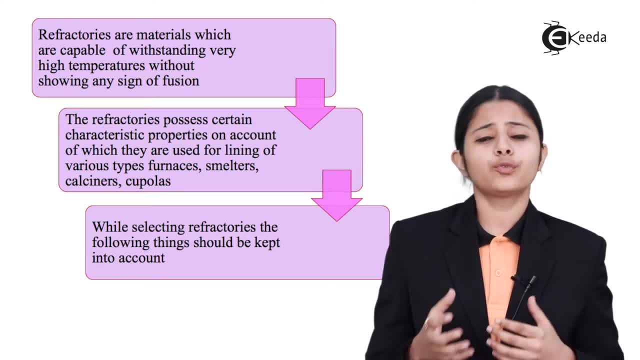 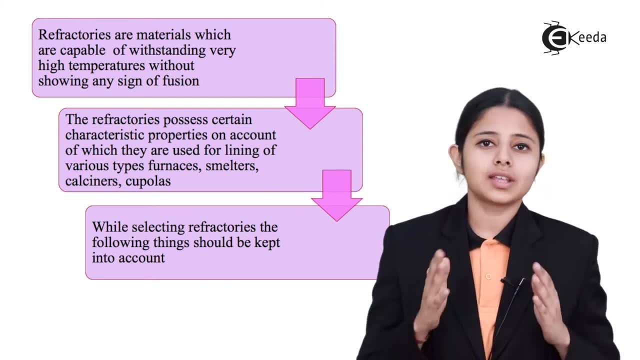 cancerners. Apart from withstanding extremely high temperature, the refractories should also withstand extremely high pressures, because inside the blast furnace there are high pressures as well. While choosing the refractories to line the internals of the blast furnace, we should keep the following properties in account. Firstly, the most important property, it should 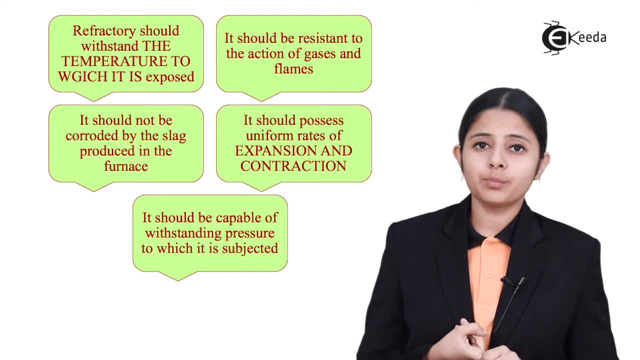 withstand extremely high temperatures. Well, the second important property is it should also withstand high pressures, because there may be many conditions and many times there are high pressures happening inside the blast furnace. Thirdly, refractory materials should be unfaced by any gases or flames which are happening inside the blast furnace. The blast furnaces are places. 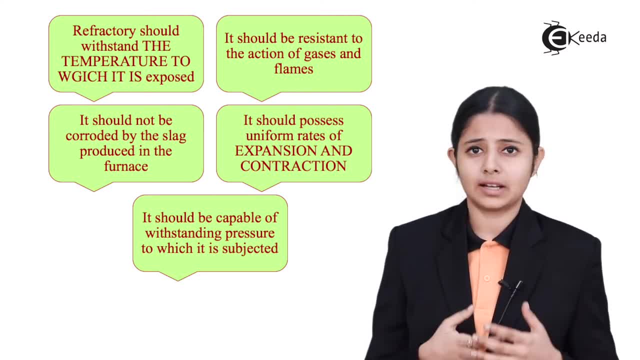 wide, open and sparse environments. However, whenever the blast furnace is active, if all the gases come into contact with the blast furnace, the degrees of fire are very low. The fire will not process the gas in the blast furnace and each time it legislators to the 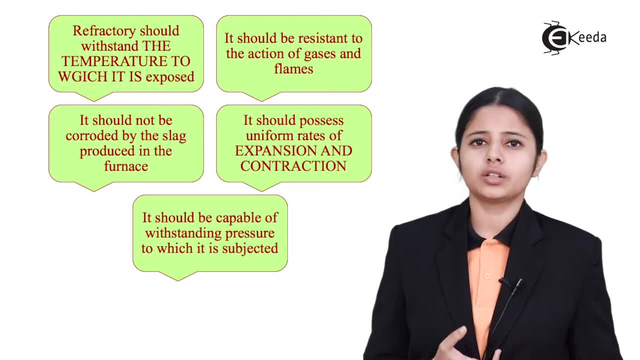 blast furnace or to the gas boilers. the gas will softens and чтобы they reheat and are suffocated. Finally, we also place the most important property of refractory materials under the place of the blast furnace, which is attached to the blowing in mucus in the 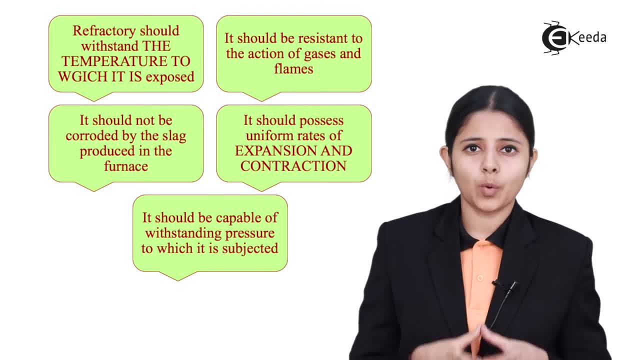 form of aила. If the Привет Fire has a flame present in the blast furnace, they are not of slag. Slag is a very important by-product which always comes out when we try to purify the metal, and if this slag combines with the refractory, 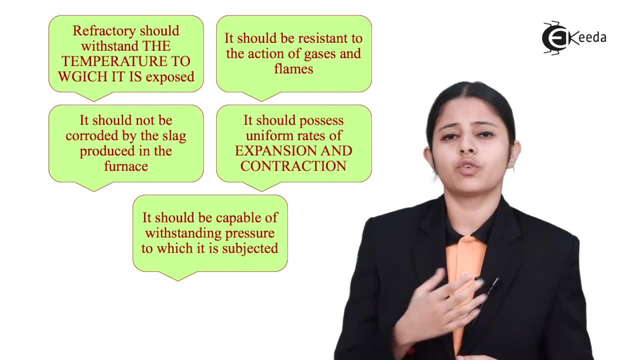 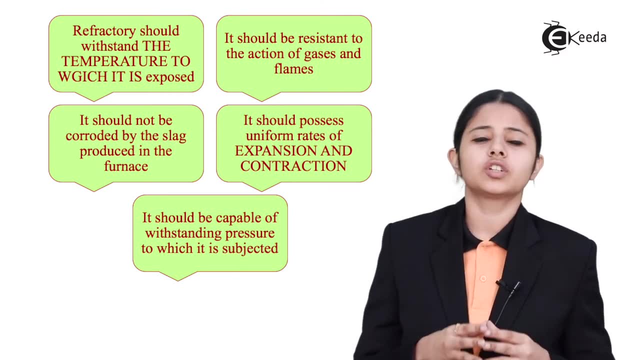 materials. it is of no use when next time we use the blast furnace for purification of the metal again. So the slag should not affect the blast furnace at all. For that the refractory material should not be any way reactive with the slag. The last very important property of the refractory materials which should be: